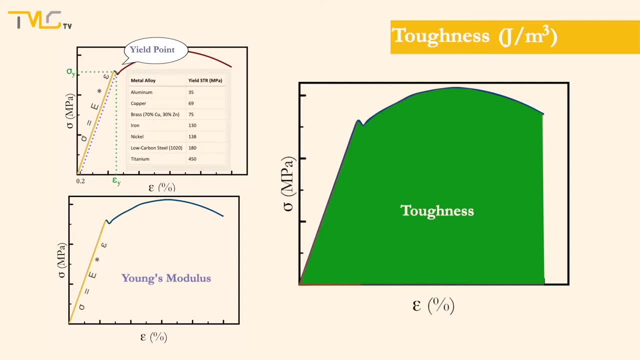 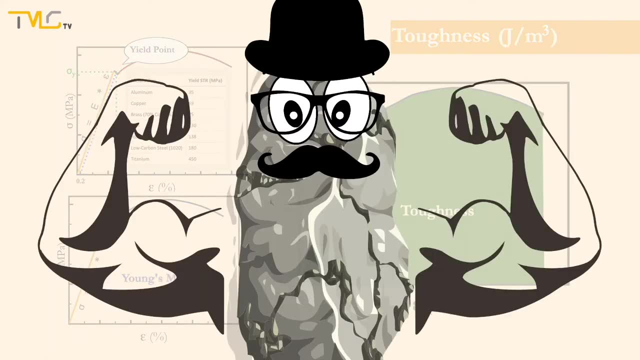 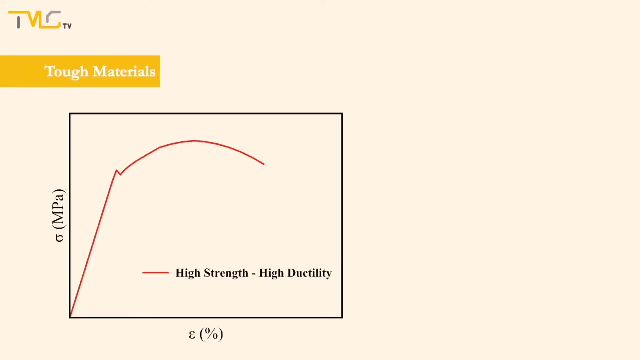 selection alongside with yield, strength and Young's modulus. Yet quantitative toughness measurements may not be very practical all the time. As a result, qualitative characteristics of tough materials are defined for a rapid classification. A material is classified as tough if, and only if, it shows both high strength and ductility. Hence most ceramics show high-strength. 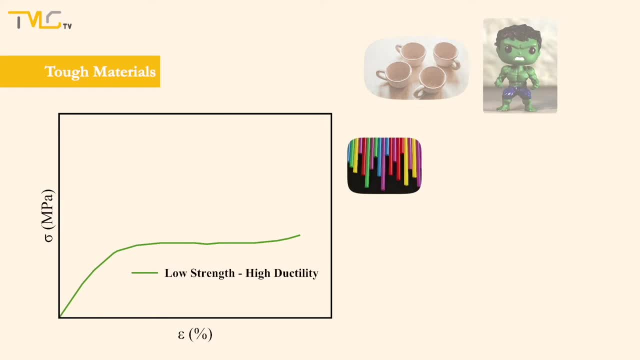 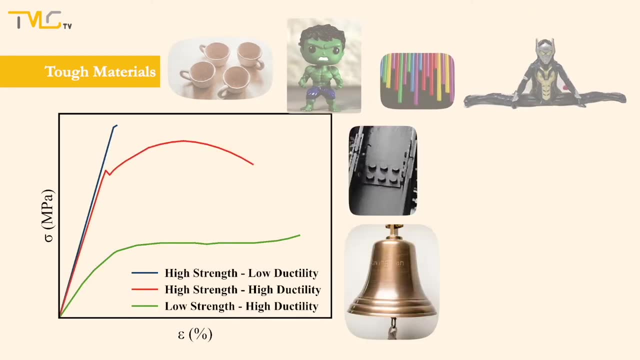 but low-ductility, and most polymers show high-ductility but low-strength. As a result, they are not classified as tough materials. Most of the metals and alloys, on the other hand, satisfy both of these requirements and are classified as tough materials. 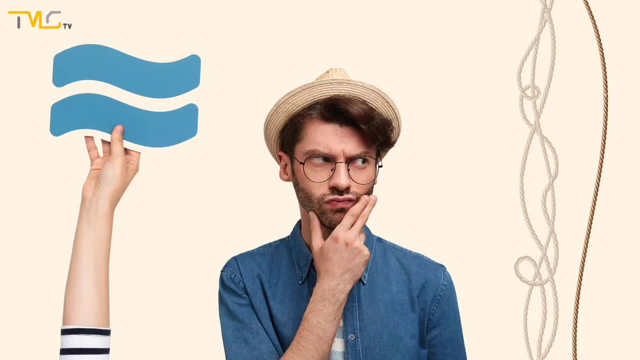 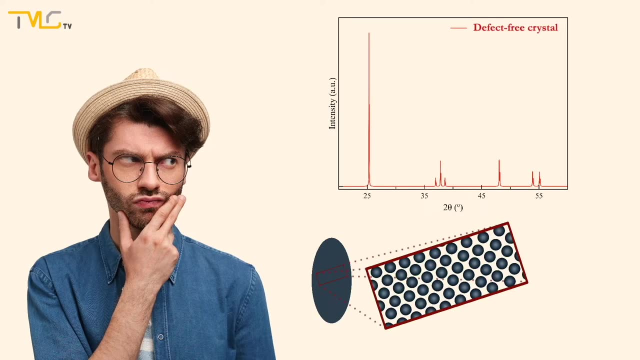 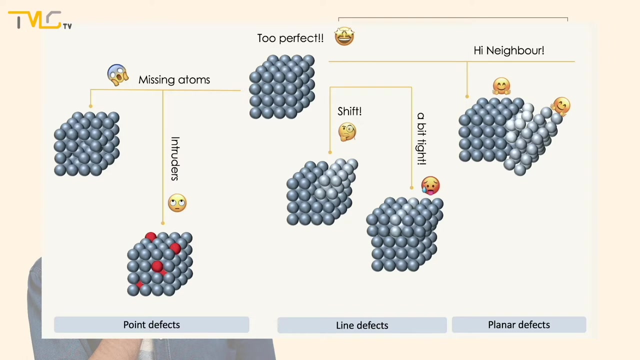 Various approximations, assumptions and simplifications can be utilized for engineering analysis. One assumption employed for mechanical analysis is specimens being defect-free. However, the theory of defect-free analysis is that the material is defect-free, As discussed in video 1.3,. in practice, it is almost impossible for a material to be defect-free, So for 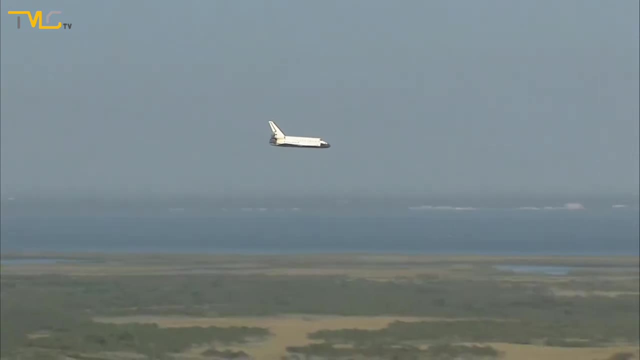 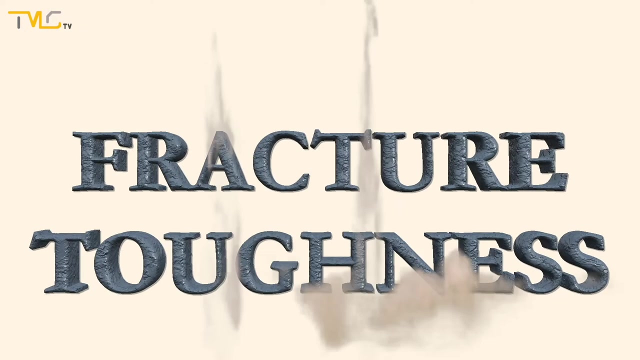 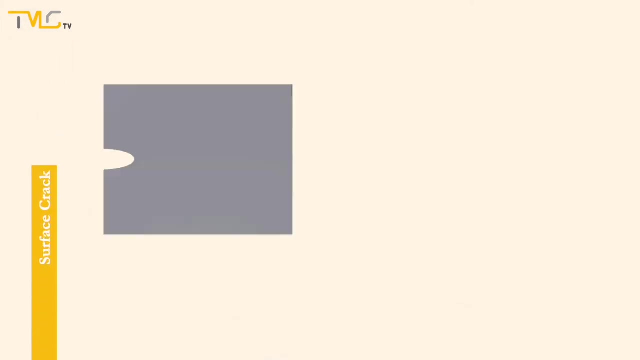 our toughness analysis to be more down to earth. we need to take the defects present in the materials into account, Which leads to the first new concept of this video, which is fracture. toughness Specimens may contain cracks on their surfaces or in their bulk volumes. Cracks are known to concentrate stress at their tips, meaning. 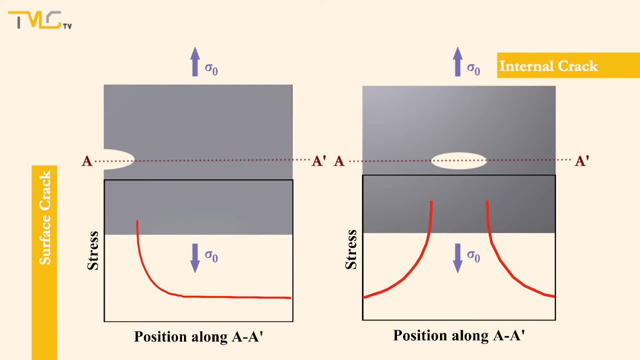 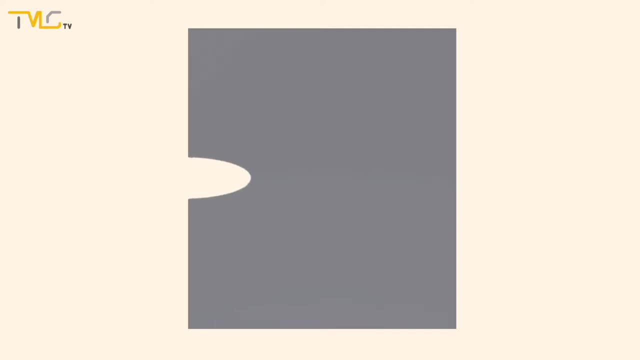 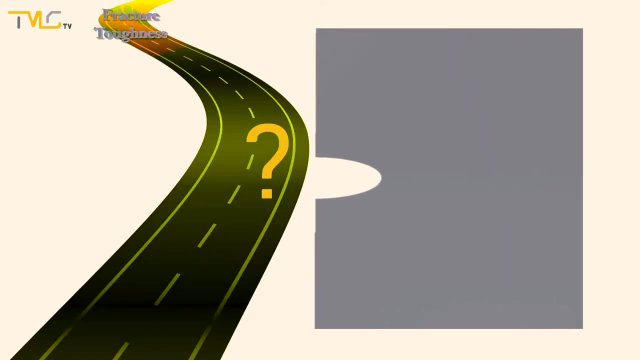 that the applied stress will be amplified due to this phenomenon, which may lead to the premature fracturing of the materials. All fracture processes go through crack formation and propagation. Therefore, before we get into fracture toughness, firstly we need to understand how these mechanisms work. Whether the fracture is ductile or brittle is significantly. 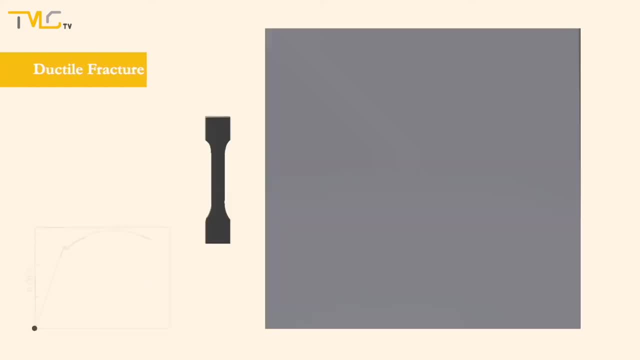 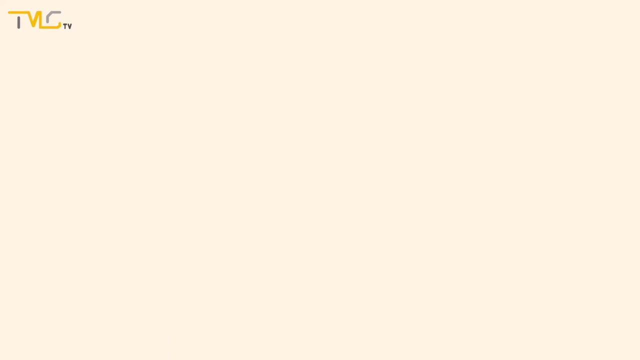 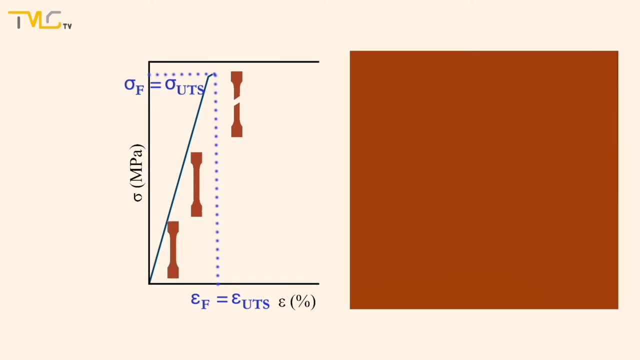 influenced by how cracks propagate During ductile fracture. a crack advances gradually, It is more stable and shows plastic deformation around itself, which prevents material from having a catastrophic failure. On the other hand, some cracks may propagate very fast and not have a lot of plastic deformation. Hence they are unstable. and once they form, 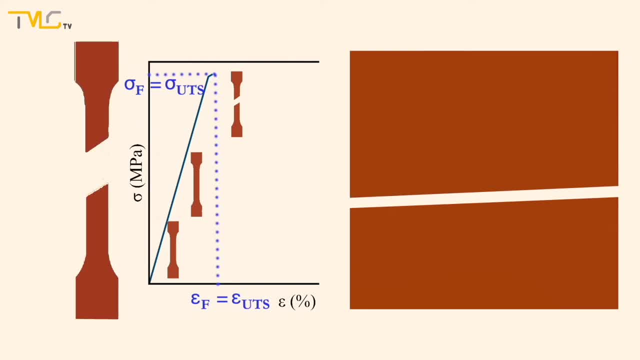 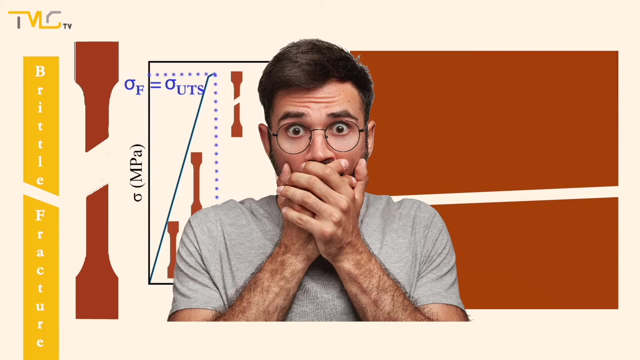 they continue propagating, even if the applied load is not increased, and eventually, but rapidly, material fractures. This type of fracture is called brittle fracture. As brittle fracture cannot be predicted or observed, brittle fracture is called as a catastrophic failure, since the fracture occurs after a rapid crack propagation. 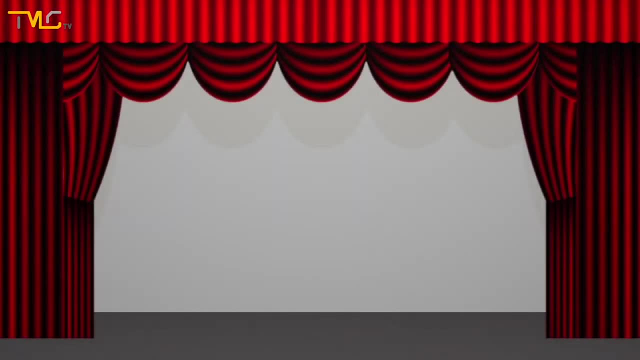 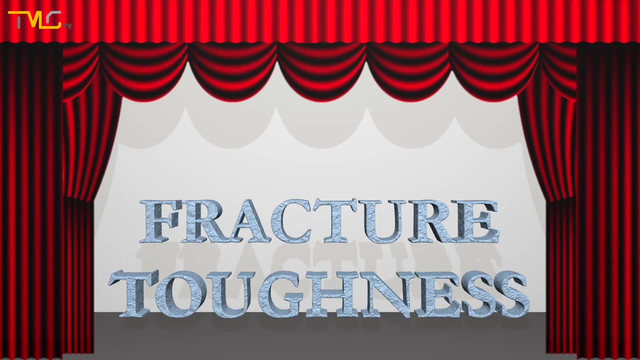 Now, with the scene set, we can go back to our second focal point: fracture toughness. Fracture toughness measures how much a material with a crack can resist brittle fracture. In other words, fracture toughness stands for the magnitude of a material's resistance. 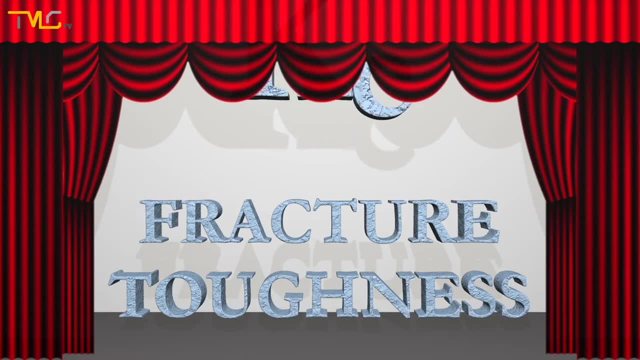 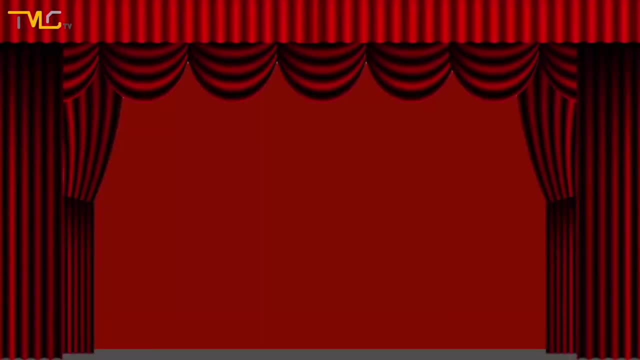 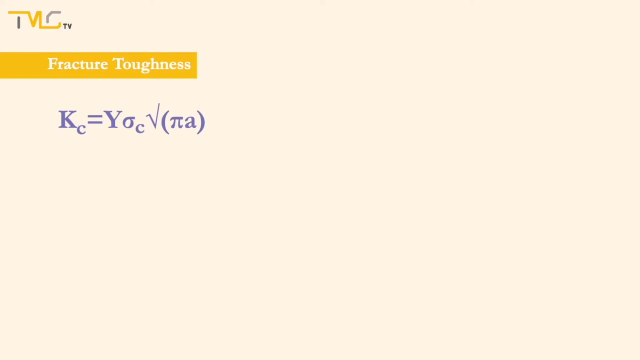 for a crack propagation. It is denoted as Kc and reported in MPa times: square root of meters. In this formula, fracture toughness is proportional to the square root of a crack length, which is denoted as A. Sigma C stands for the critical stress of crack propagation and its equation. 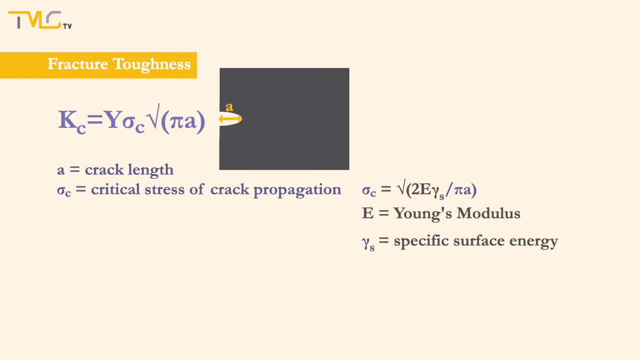 is given on the screen. Y is a dimensionless correction factor used for taking the size and geometries of a fracture, cracks and specimens and type of applied load into account. Sample thickness has a profound effect on fracture toughness for thin samples, yet as 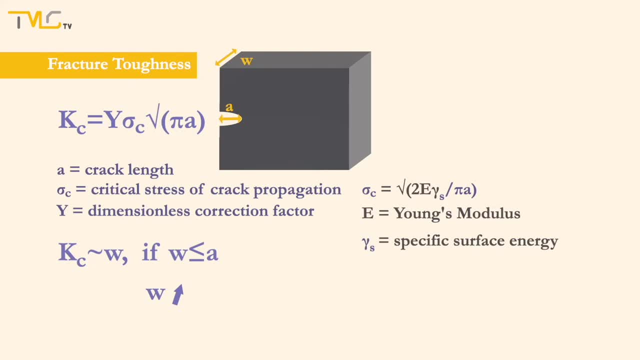 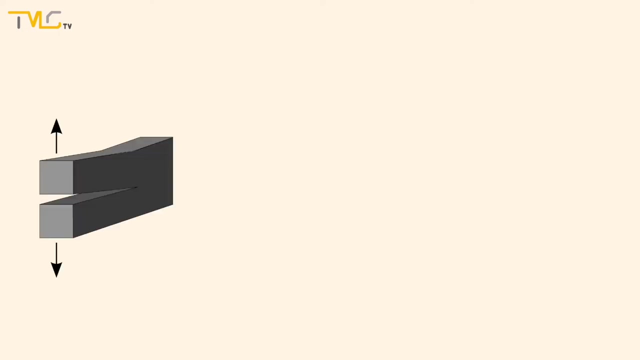 the sample thickens, its influence on fracture toughness decreases and beyond the certain thickness threshold, fracture toughness becomes independent of the sample thickness. For the cases where strain occurs only on the loading plane of thick samples, we obtain plain strain fracture toughness denoted as K1C. 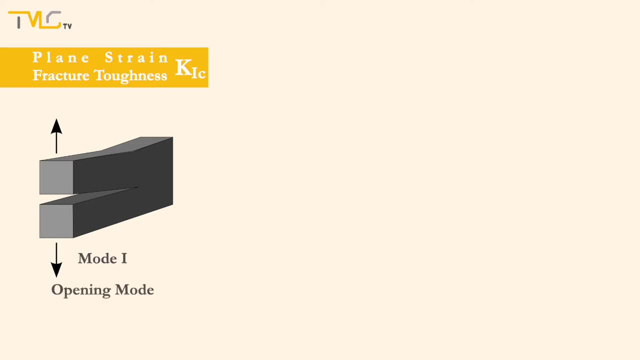 One in this notation shows the mode of crack displacement, which is named as opening or tensile mode. There are also types 2 and 3 that are called sliding and tearing modes, and they won't be covered in this video. A brittle material will not go through a 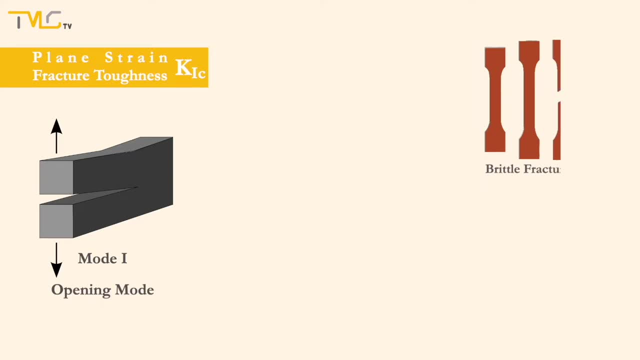 contraction. A brittle material will not go through a contraction. A brittle material will not go through a contraction. K1C will have a considerable amount of plastic deformation. hence it will have a low K1C value. that may lead to a catastrophic failure. 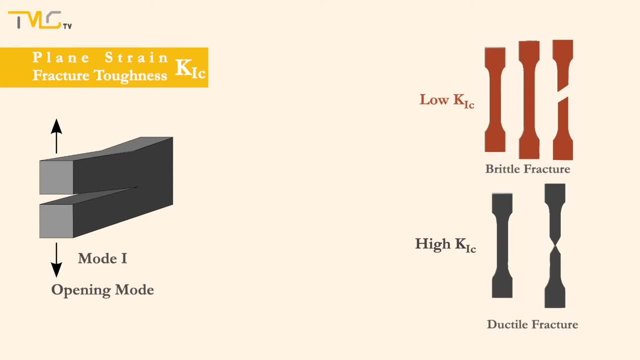 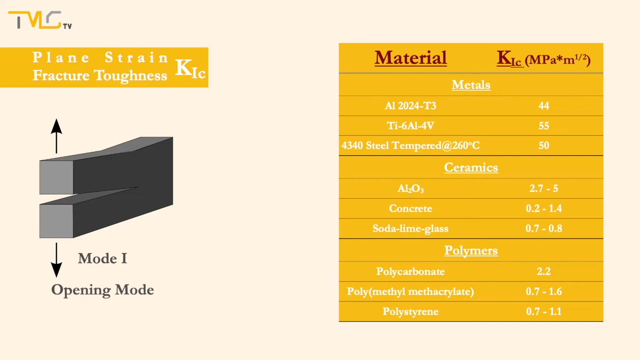 Oppositely ductile materials have larger K1C values as they show high strength and go through a comparatively large amount of plastic deformation. K1C is employed to determine whether a material will undergo a catastrophic failure or not. K1C of a material strongly depends on the temperature, strain rate and microstructure. 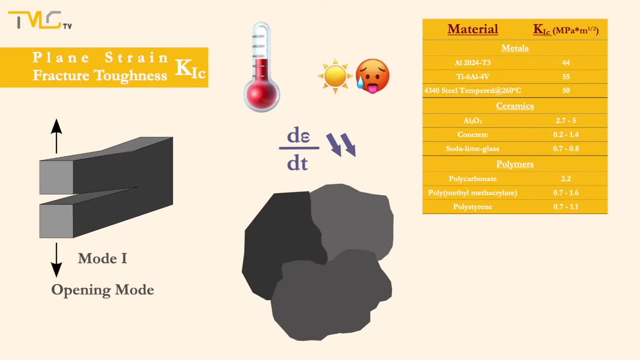 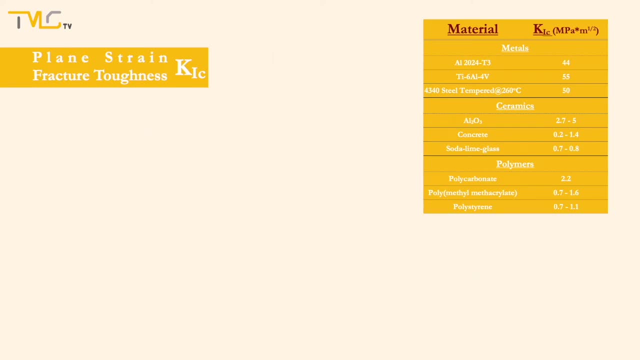 microstructure. Thus, higher temperatures, lower strain rates and finer grains promote higher K1C values. Fractured toughness is one of the major parameters employed when selecting a material for a mechanically demanding application. In this context, fractured toughness is employed for deciding the maximum. 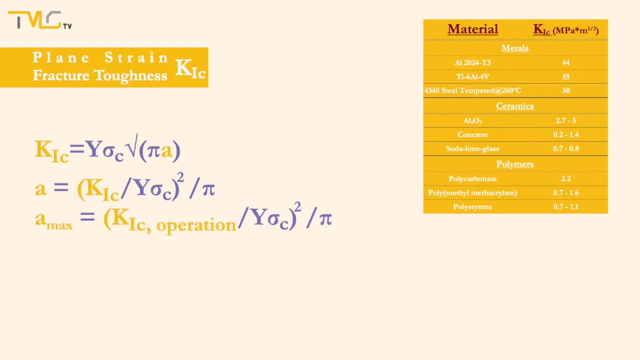 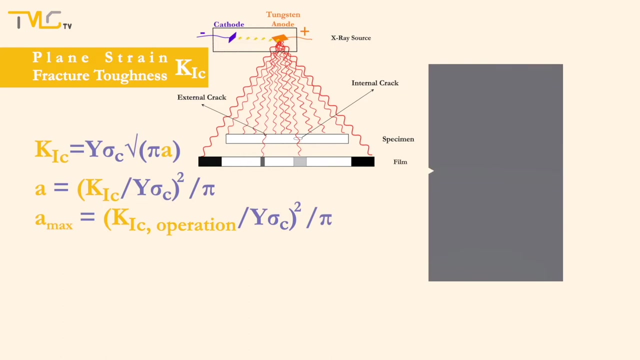 allowable crack size on material to prevent a catastrophic failure under operation. The internal and external cracks on the specimen can be detected by a non-destructive testing method called radiography. Yet for fractured toughness testing, a specimen with a carefully machined, sharp crack on it is used. These tests are performed at a constant loading. 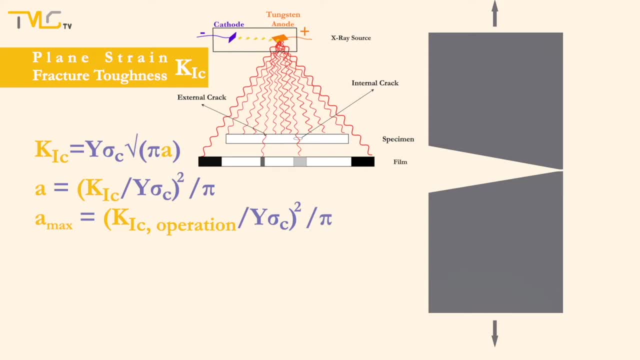 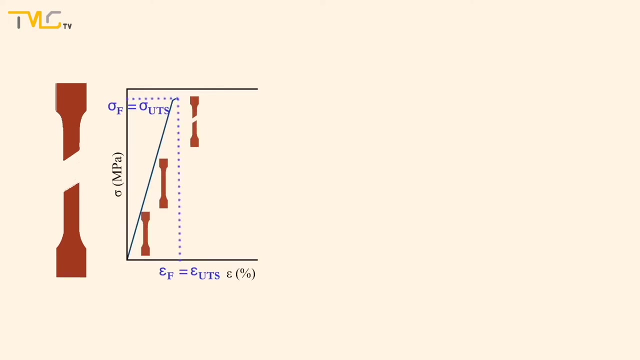 rate. Then the collected load and crack displacement data are evaluated and obtained. results are employed for fractured toughness analysis A. As said in the beginning of this video, some materials fracture suddenly with little or no plastic deformation. For such cases, impact testing techniques become handy for evaluating the mechanical 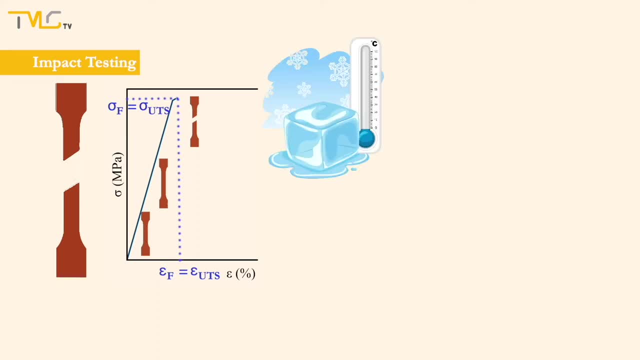 properties of materials under severe conditions such as low temperature, high strain rate and triaxial stress state. Two standardized impact testing methods are Charpy and Izot. These tests are quite similar. the main difference between them is the orientation of the specimen. 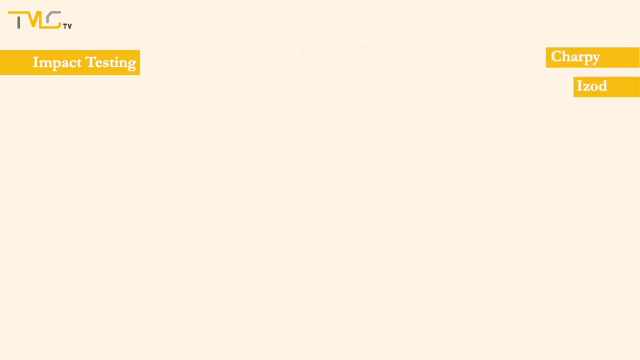 in the test apparatus, V-notch of the sample is positioned perpendicular to the floor for Charpy and parallel to the floor for Izot testing. For both of these techniques, a square or a rectangular prism specimen having a V-notch machined in the middle is placed on the setup. 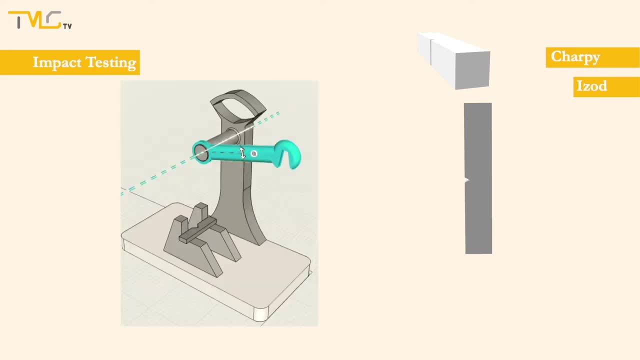 Then a weight pendulum hammer is released from a fixed height for an impact blow, loading on the specimen. As the hammer hits the back of the specimen, some of the energy is absorbed by the specimen, leading to the fracture of it from the stress concentration point at the V-notch region. 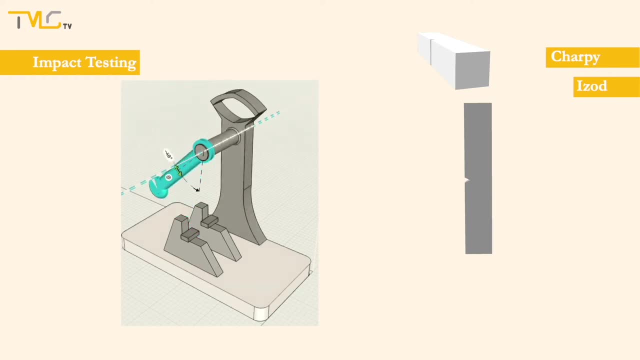 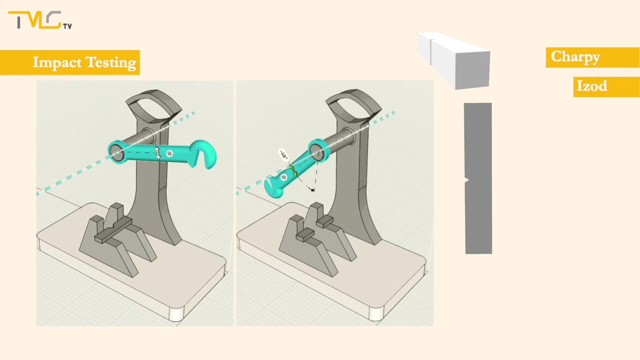 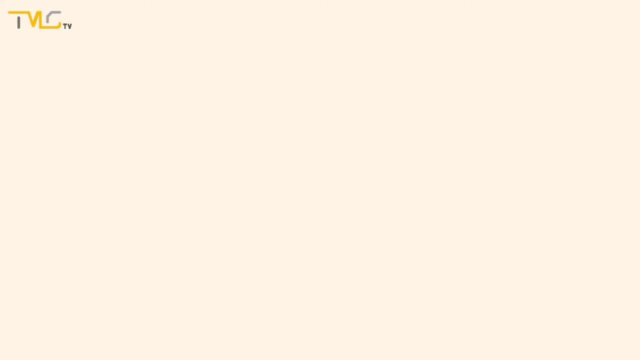 After the fracture, the hammer rises up to a certain height which is lower than the initial one. This height difference gives the amount of energy absorbed by the specimen during fracture and is called the notch toughness of the specimen. Charpy and Izot tests become very useful for determining whether a material has a ductile-to-brittle. 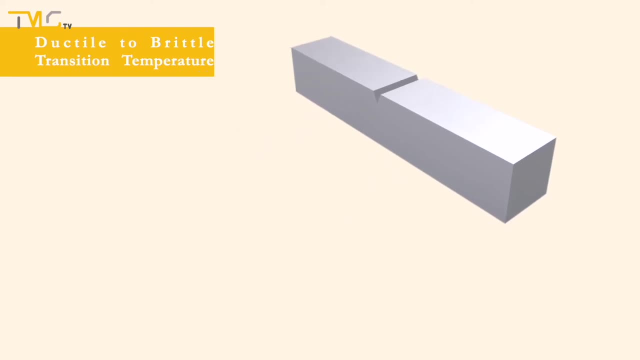 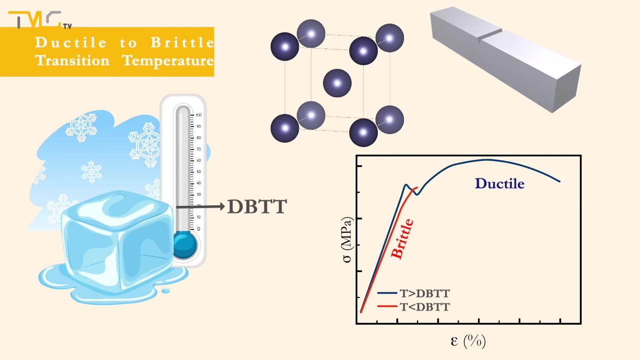 transition temperature or not. Ductile-to-brittle transition is a phenomenon observed for metals with BCC structure. As such materials are cooled below a specific temperature, which is called the ductile-to-brittle transition temperature, their mechanical behavior changes from a ductile one to a brittle one. 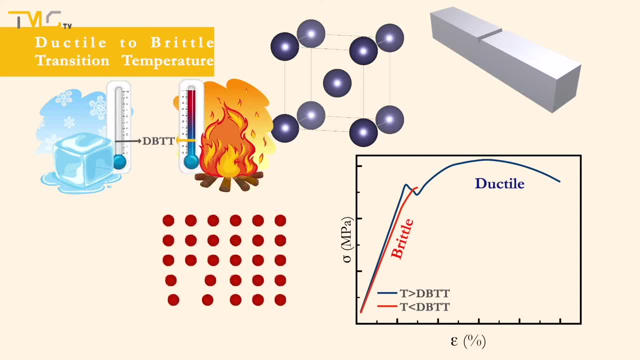 The dislocation motion of BCC materials highly depend on the temperature. Thus, at high temperatures, dislocations are mobile, resulting in a ductile behavior. However, As the temperature decreases, the dislocation mobility drops as the number of available slip systems decreases. 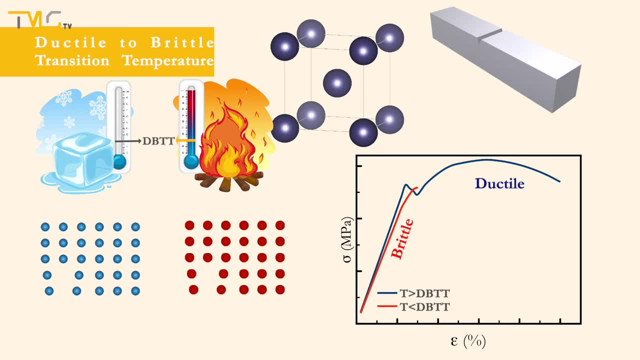 And as the temperature reaches below ductile-to-brittle transition temperature of the material, dislocations become immobile, which makes the material to show brittle fracture characteristics. Ductile-to-brittle transition phenomena is not observed in FCC structures, since they 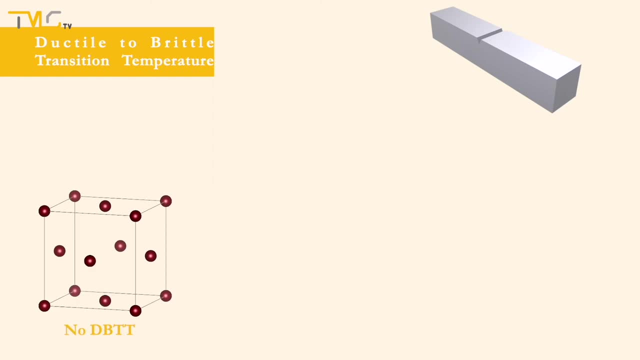 have many slip systems for dislocations which can be activated with low energies. Also, The strength materials are brittle at all temperatures. therefore we cannot talk about a ductile-to-brittle transition for them. Ductile-to-brittle transition temperature can be determined by Charpy anisotests, while 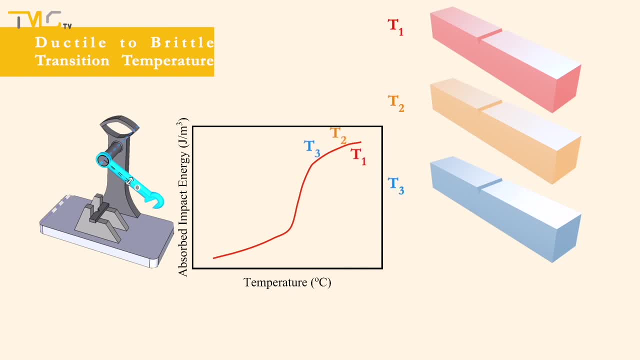 testing the same material at various temperatures. If a specimen shows a drastic decrease in notch toughness below a certain temperature, this means that the specimen shows ductile-to-brittle transition. Then A new set of temperatures can be selected around the temperature of the ductile-to-brittle. 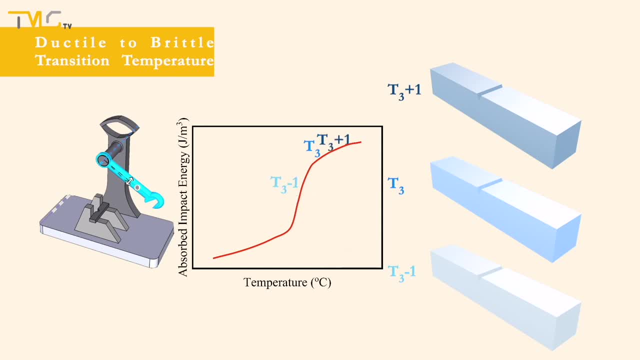 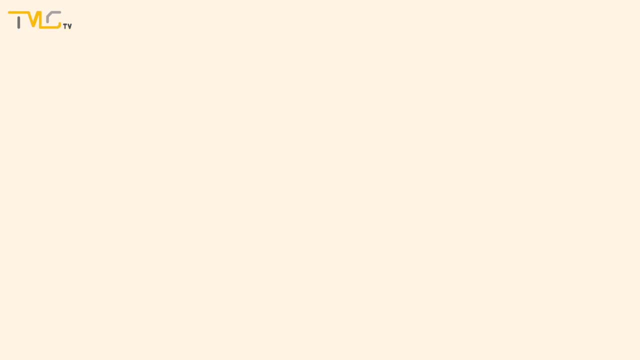 transition. This means that the specimen shows ductile-to-brittle transition. However, where this behavior is observed, to pinpoint the ductile-to-brittle transition temperature precisely To determine the fracture characteristics of a material, both plane strain, fracture toughness and notch toughness can be used.